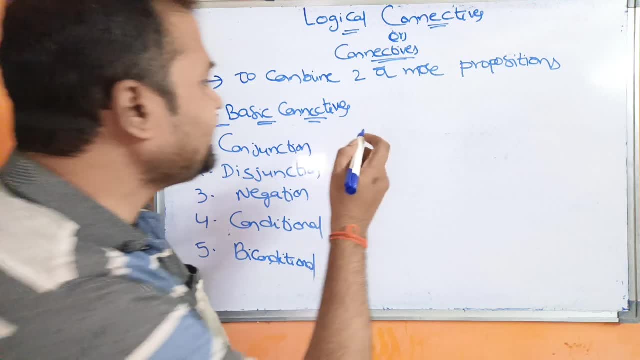 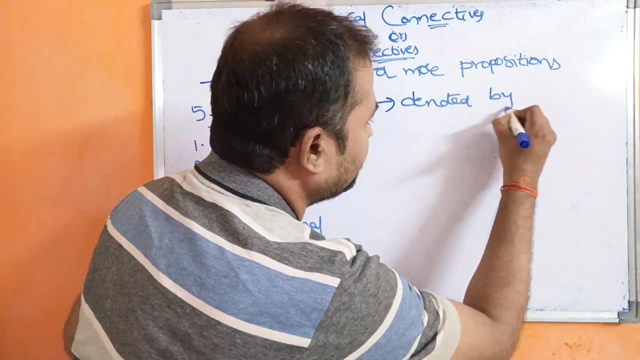 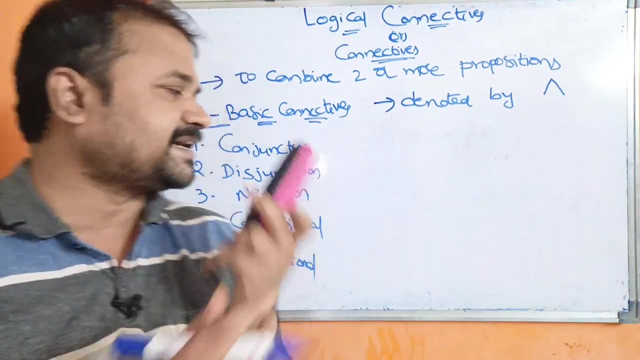 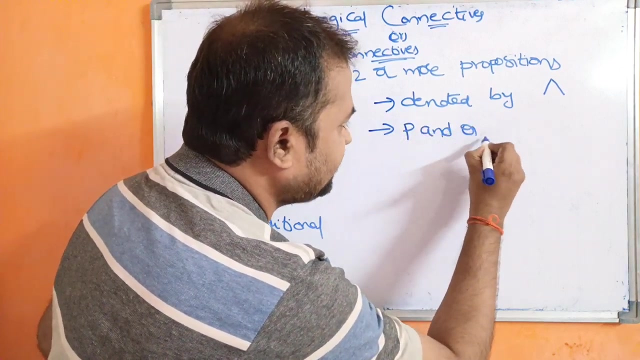 one is conjunction. Conjunction is denoted by the symbol and Conjunction is denoted by which symbol and symbol And means inverse of V. Let us see what is conjunction. Let we have two prepositions, such as P and Q, Then the conjunction is denoted. 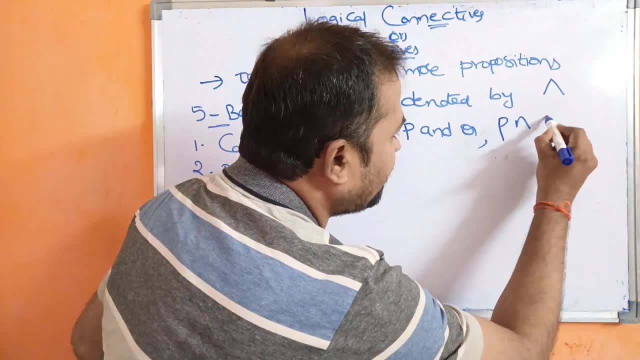 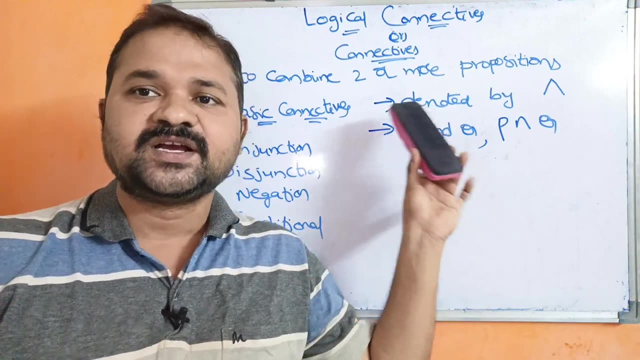 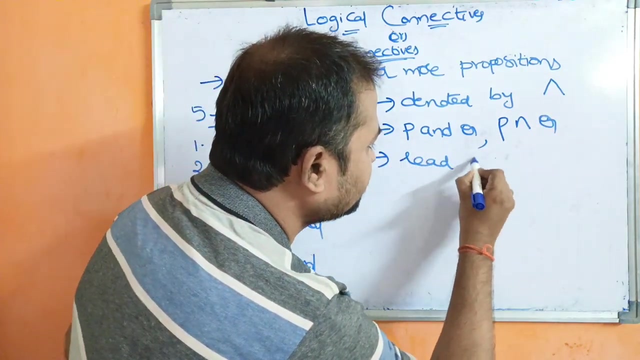 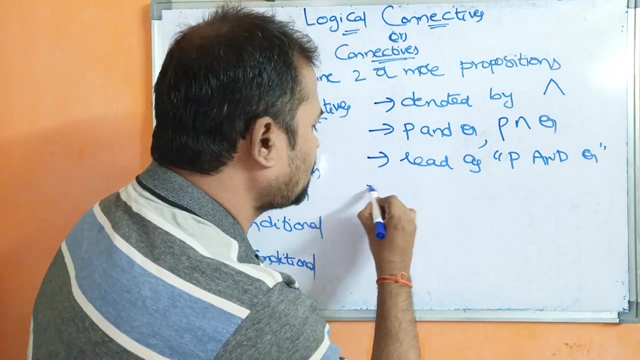 by P and Q. If there are two prepositions such as P and Q, Then the conjunction of two prepositions such as P and Q is denoted by P and Q, And P and Q is ready as, Which can be ready as P and Q. Now let us see what is under operation. P and Q returns- true Returns. 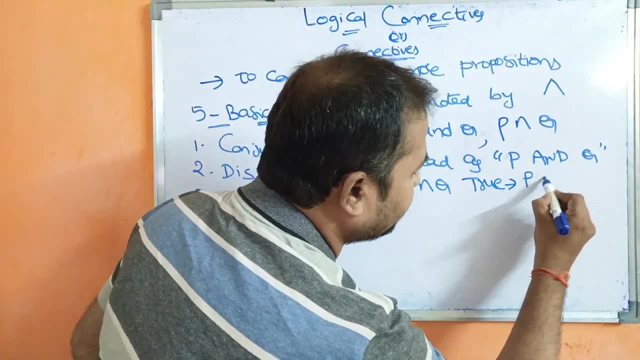 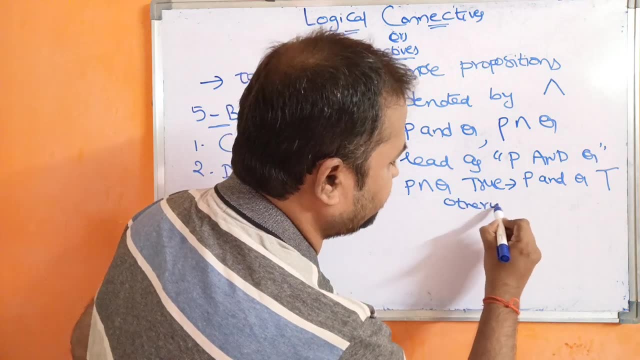 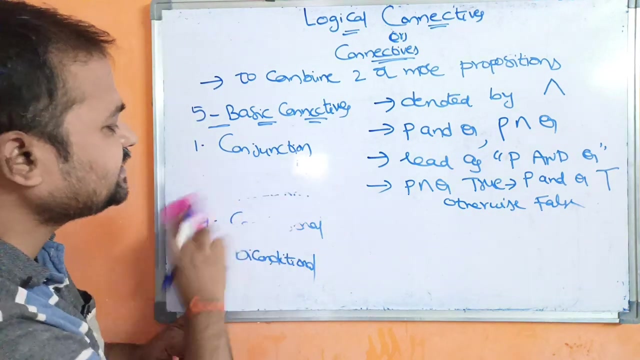 true When P as well as Q is true. Otherwise, it will returns false. Now let us see what is under operation. Now let us see what is under operation. P and Q returns true When P as well as Q is true. False value. Otherwise it will returns which value False value. So let us see the 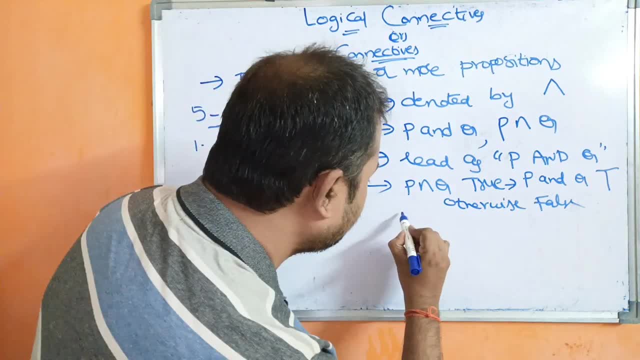 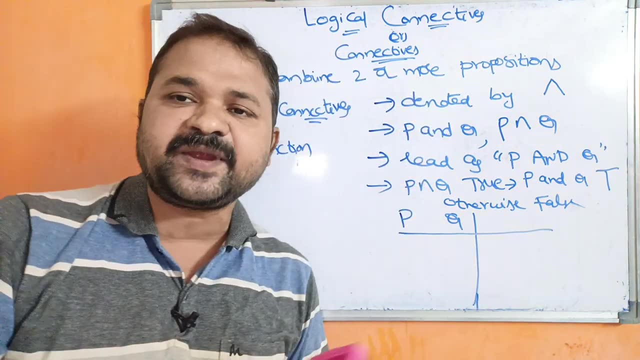 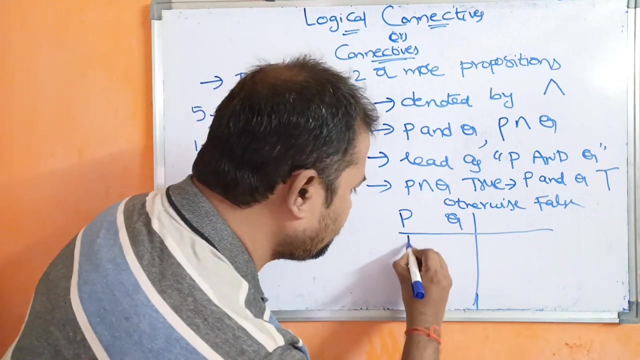 truth table here. Let us see the truth table. So this is P, This is Q. We have two prepositions, are there? If there are two prepositions or statement, Then totally two power, two combinations are possible. Why? Because two prepositions are there. So the possible combinations are: 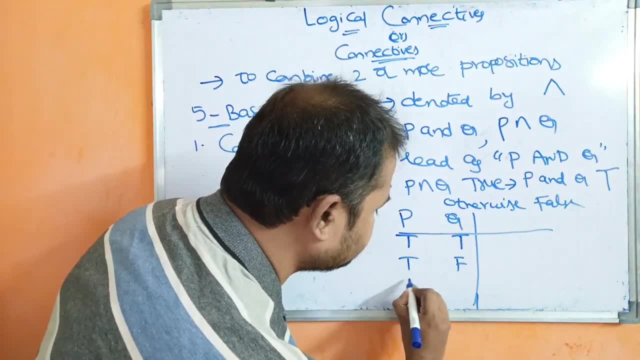 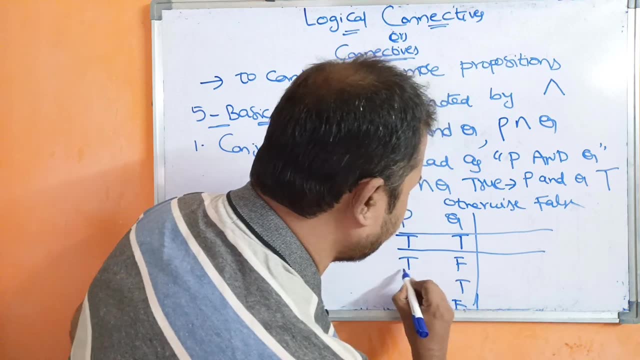 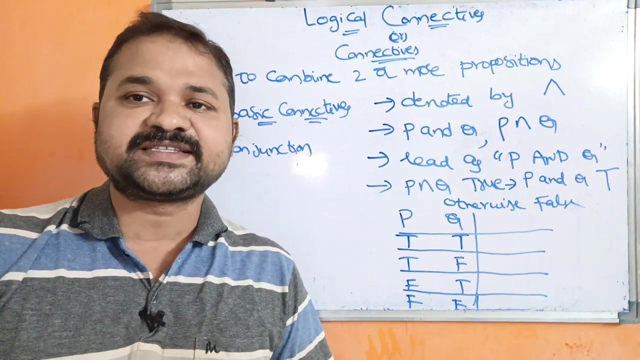 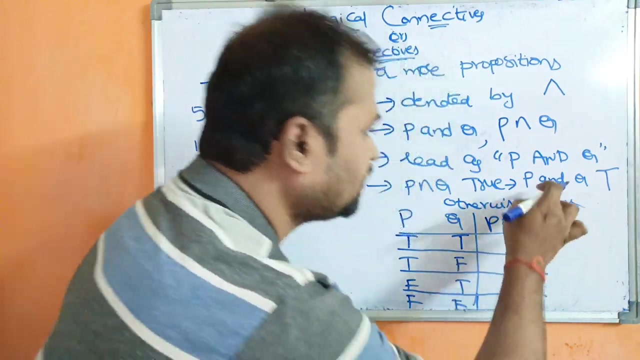 true, true, True, false, False, true And the last combination is false, false. So true, true is the first combination, True false is the second combination, False, true is the third combination, Whereas false, false is the last combination. P and Q is true when it is true If both P and Q are. 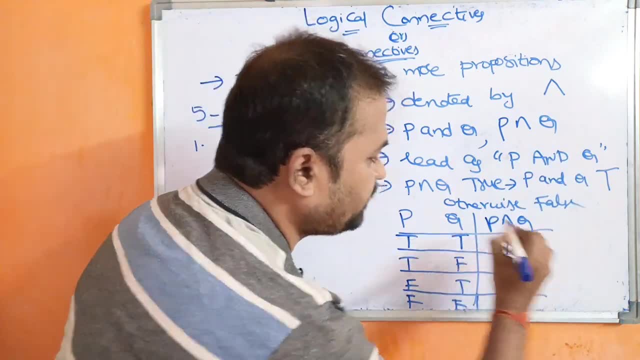 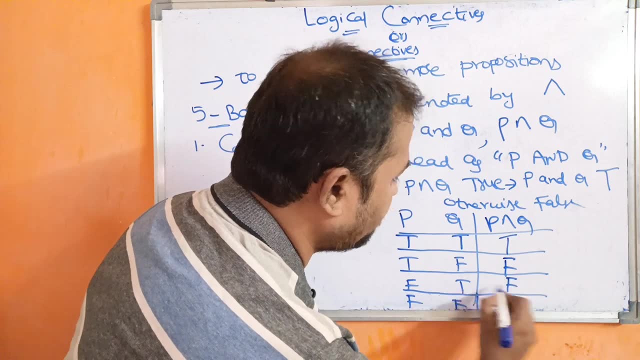 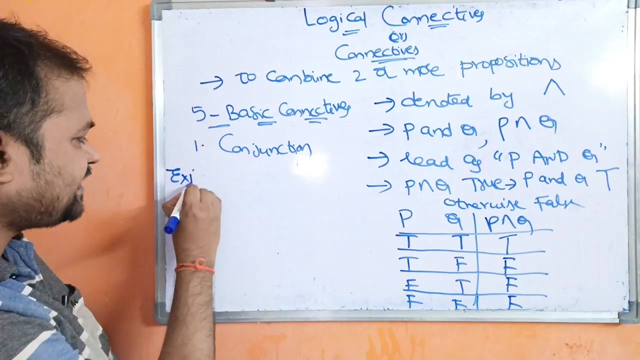 true Here, P is true, Q is true, So P and Q is true. Otherwise the result is false, So false, so true. true means true, true, false means false, false, true means false, false, false means false. now let us see some examples. let the first example is like this: it is raining. 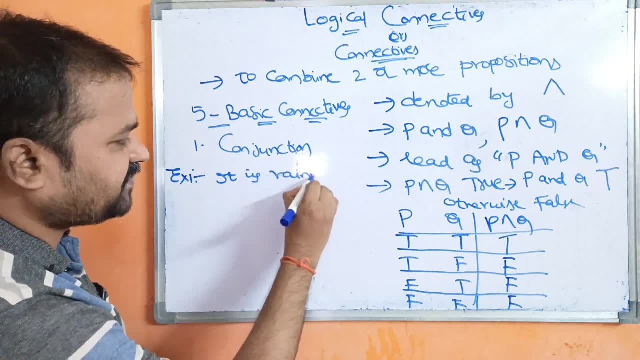 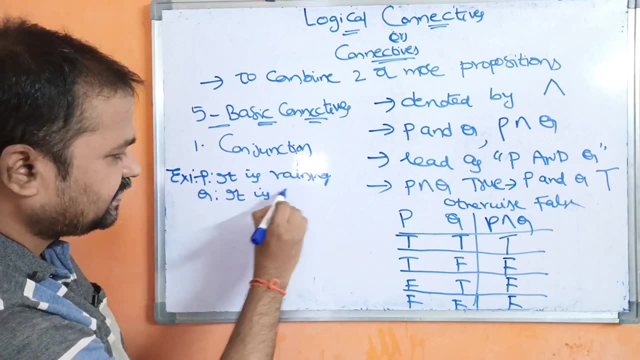 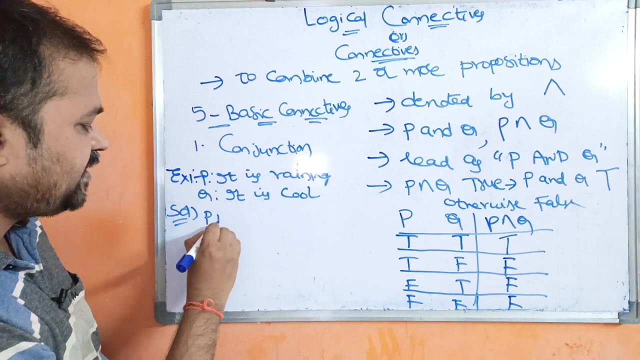 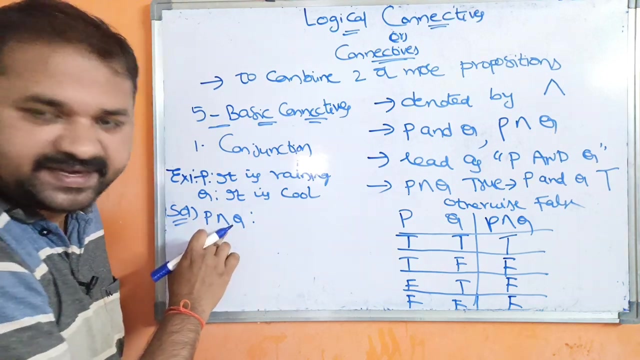 it is raining. this is the first preposition: p colon, let. the second preposition is like this: it is cool. it is cool, then, how we can write p and q, so how we can denote p and q, so p and q colon. this is the new preposition, which is obtained by uh and operator okay conjunction. 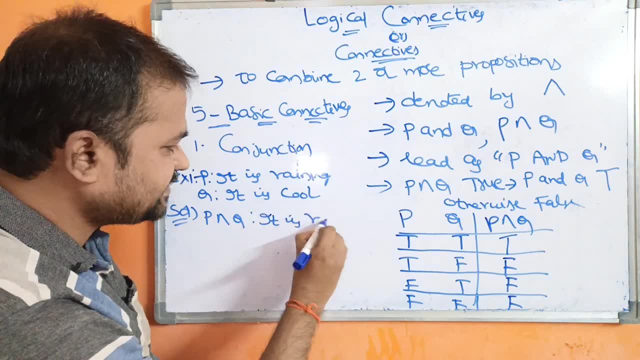 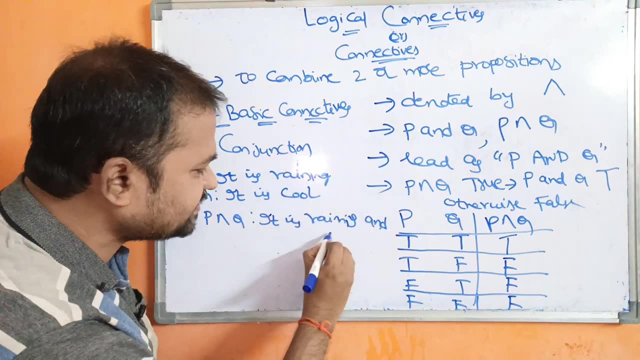 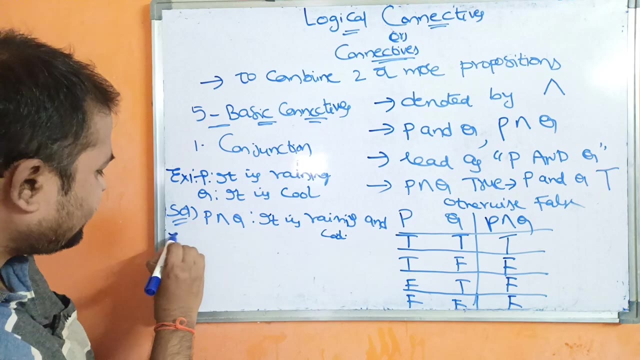 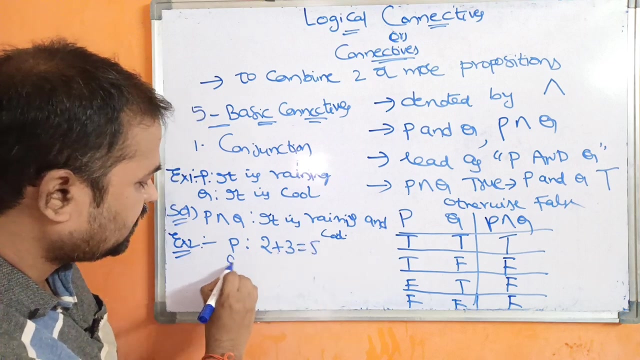 it is raining, it is raining, so conjunction means we have to use and and it is cool, it is not necessary. we can write here, school, it is raining and cool, so we can write like this: let us take the second example, example two. let the second example is like this: two plus three is equal to five. uh, let the first preposition is: 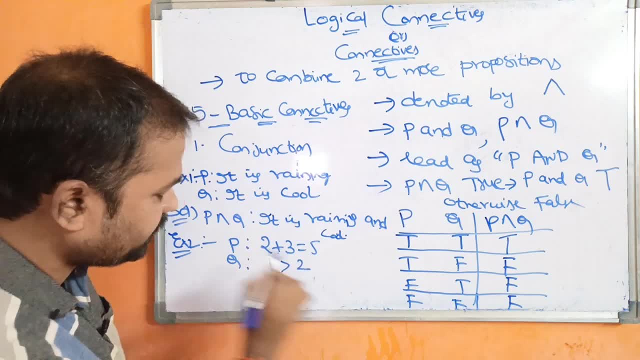 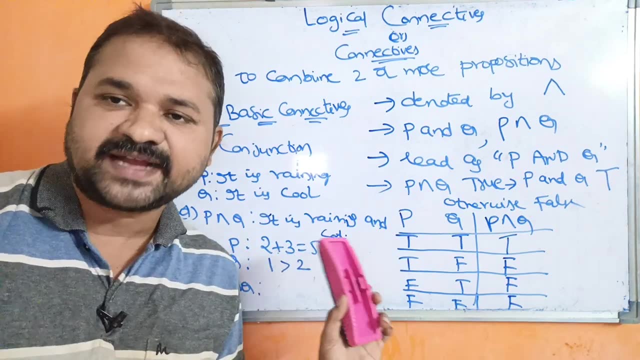 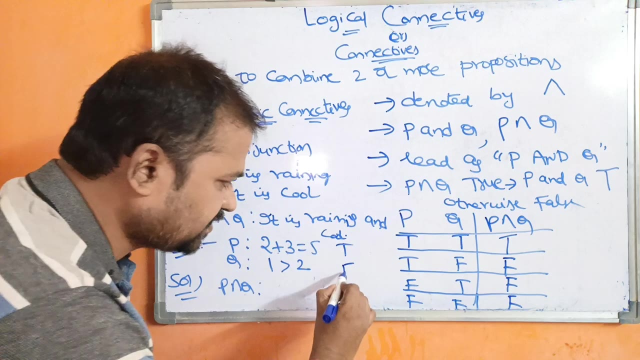 like this. let. the second preposition is like this: one greater than two, then what is the solution? p and q is two plus three is equal to five. condition is true. okay, so this is true. one greater than two. two condition is false. so true. false under operation means what true? false means false. 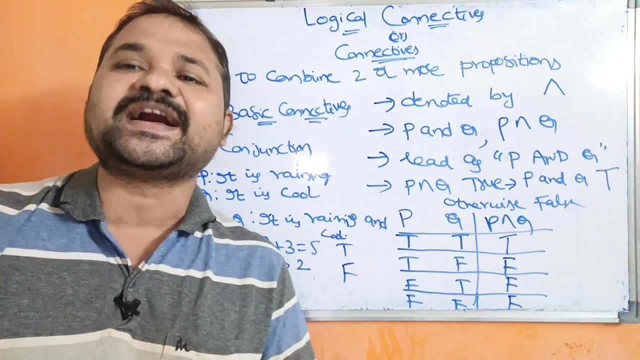 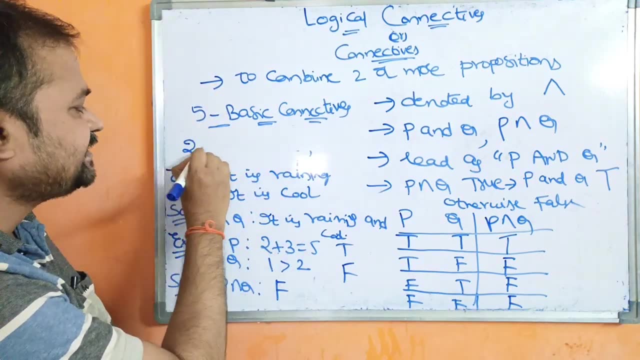 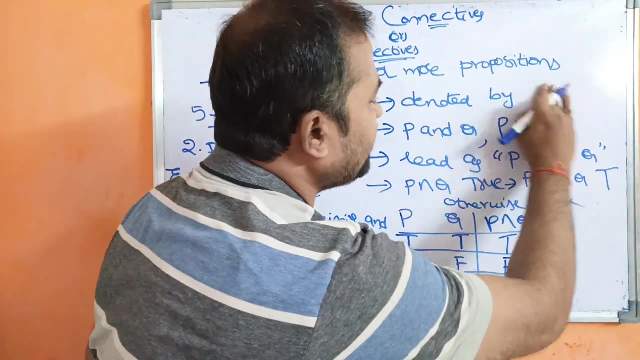 so here the result is false. so this is about conjunction. let us see the next connective, that is dissension. let us see the second one, that is dissension, dissension, dissension, dissension, is denoted by a symbol called v, so v means r. other name for the conjunction is: 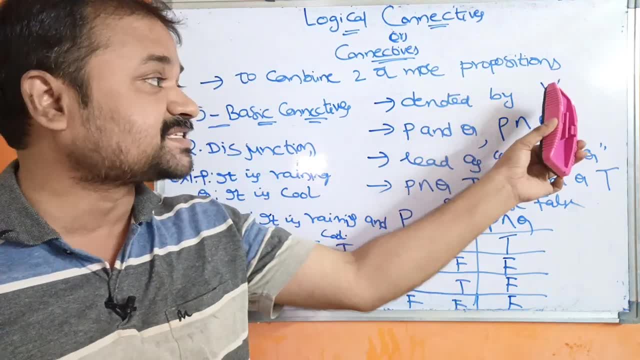 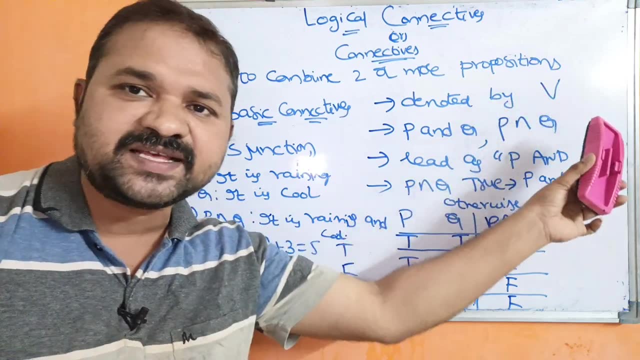 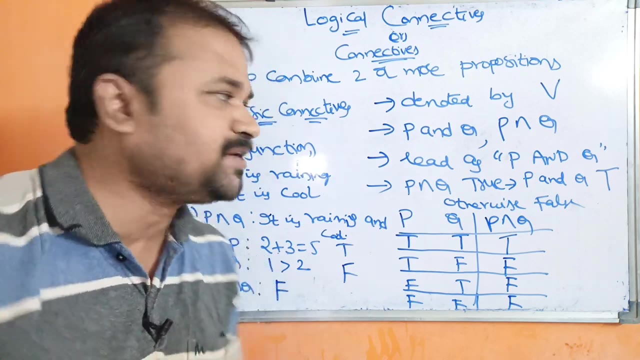 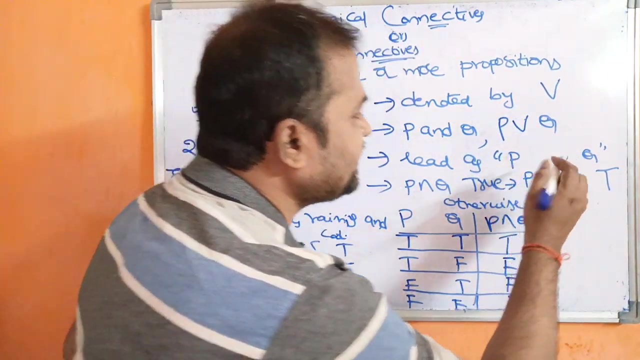 and various other name for the dissension is r r. okay, uh, it is denoted by the symbol r. dissension is denoted by the symbol r. if p and q are two prepositions, then the dissension of p and q is denoted by p r q. which is really as? which is really as p r q? it is our choice, we can use. 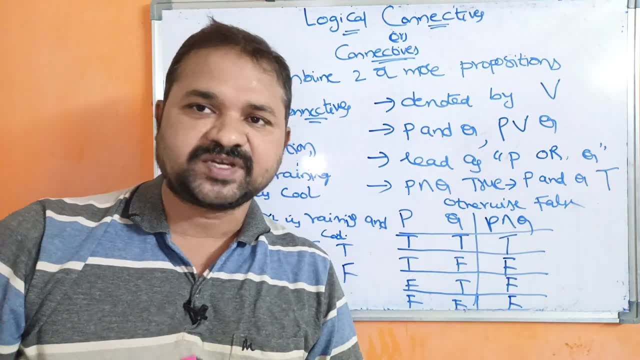 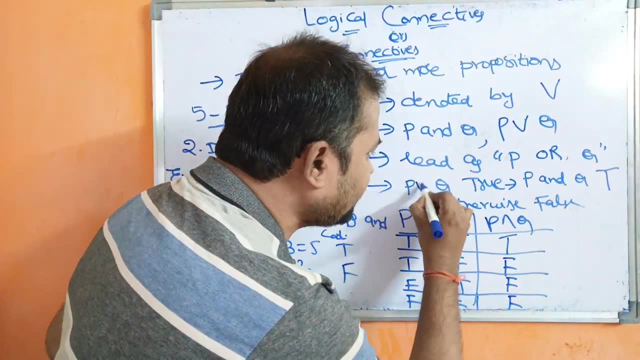 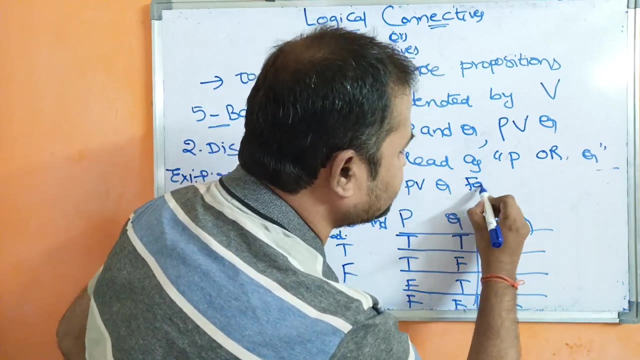 lowercase letters or uppercase letters or lowercase letters or uppercase letters or uppercase letters are combination of both, there is no problem. uh, so which can be read as p or q. let us see when it will return true and when it will return false. p and q written false. p and q written false when. 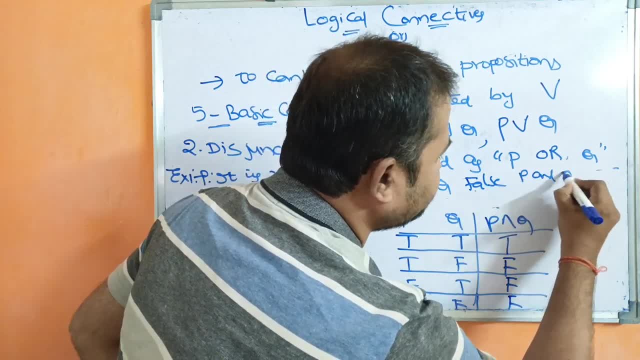 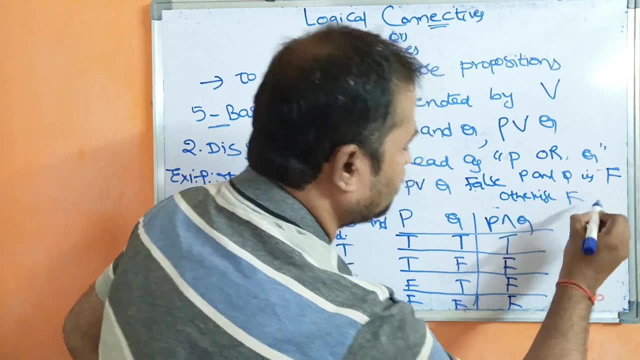 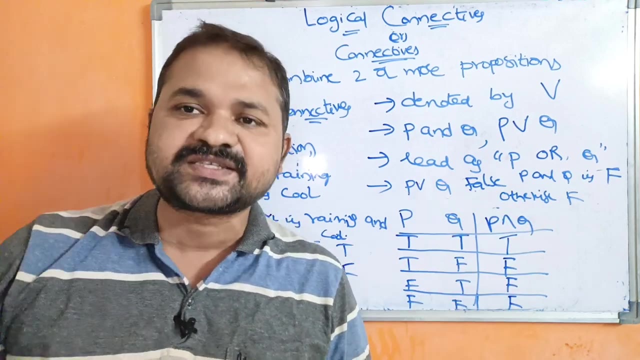 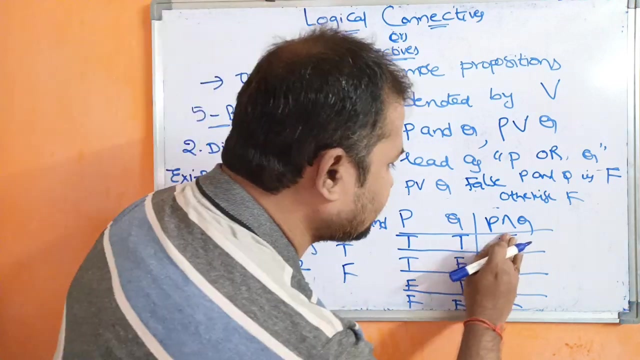 when p and q is false, when p and q is false. otherwise it will returns true. p and q is false. otherwise it will returns true. p and q is false when both p and q are false, otherwise it is true. that means if one of the preposition is true, then the result is true. so let us write the combinations here. so here false. 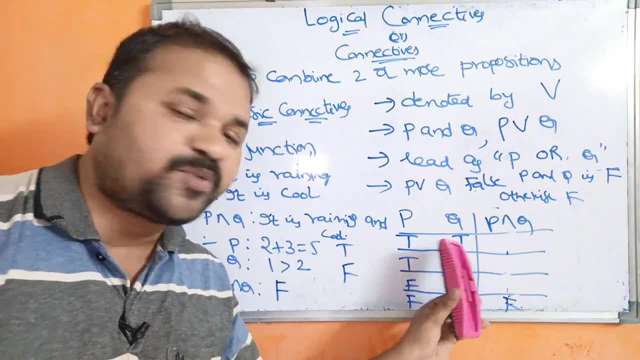 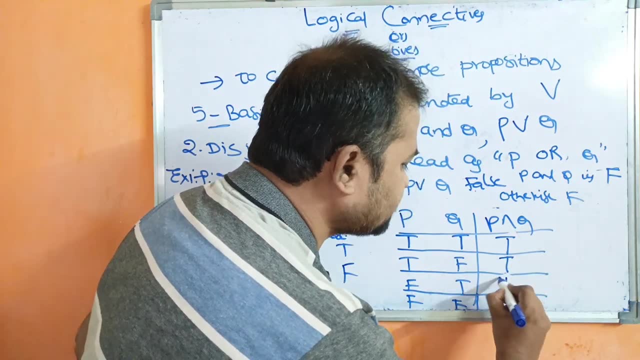 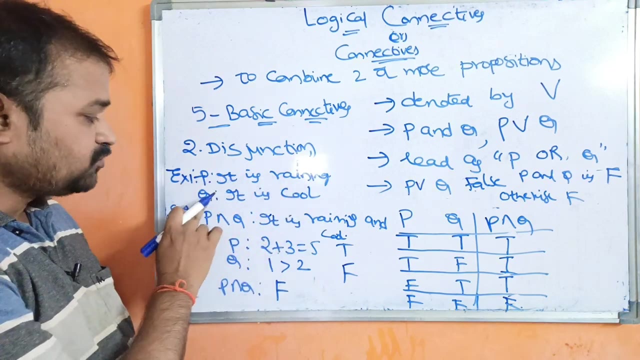 false means false. when one of the preposition is true, then the result is true. only so true. true means true. true, false means true. false, true means true. now let us see an example here. let's see the first example. it is raining. this is p preposition, q preposition. it is cool, then we can return as p. 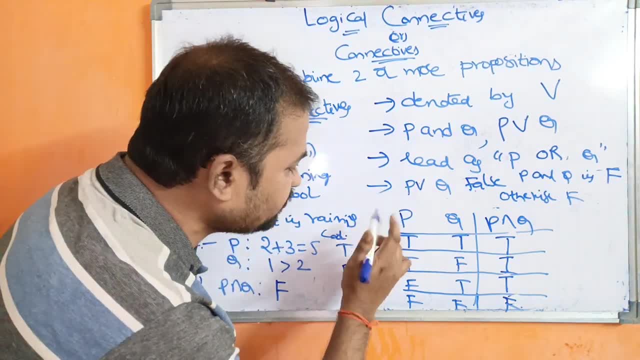 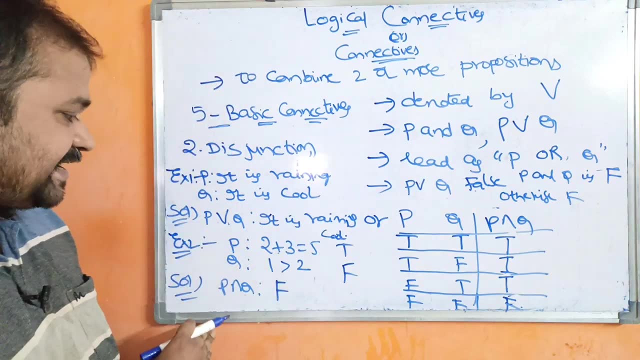 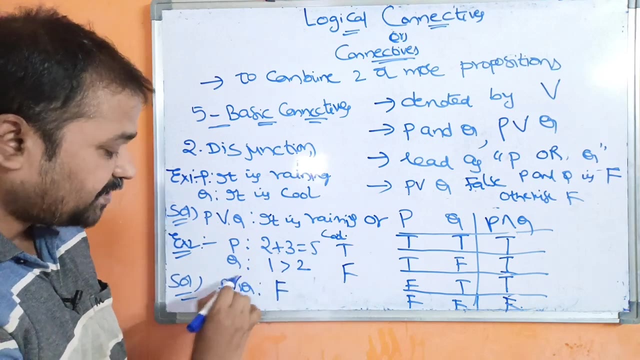 or q means it is raining. here we have to use a word called r, or it is cool or we can write as cool. that is enough. let us see the second example here. the first preposition results true value. second preposition results: returns false value. so p, r, q, so true false r. operator means what? 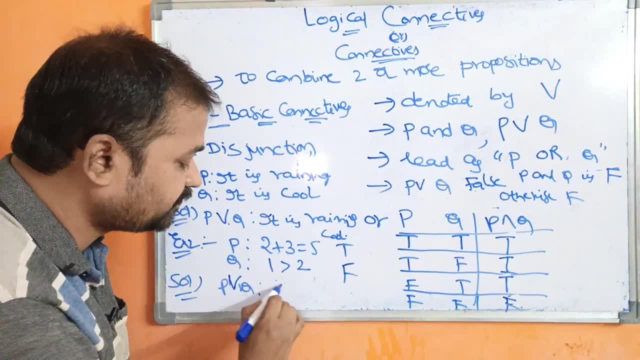 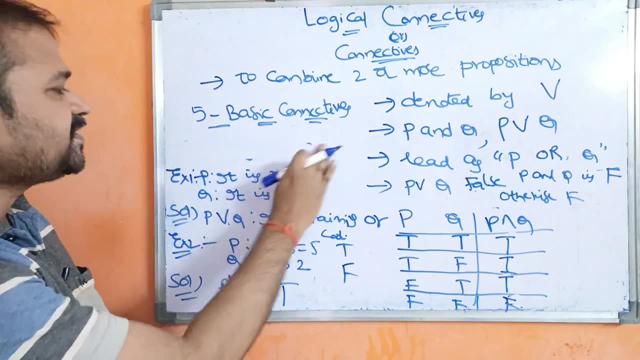 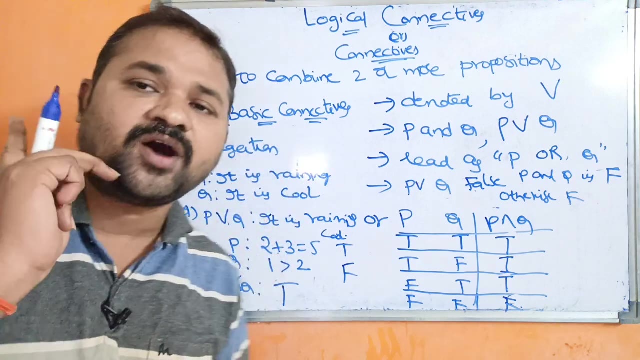 true. false means true only. So here the result is true. So this is about dissension. So dissension means R operator. Now let us see the third one. So what is the third one? Negation. Here negation is applied on a single preposition, on a single statement. Negation is denoted by three symbols. 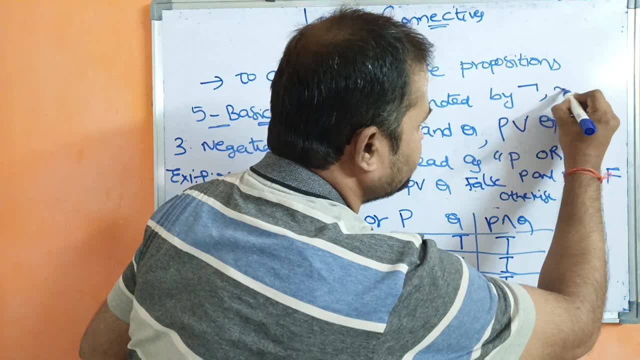 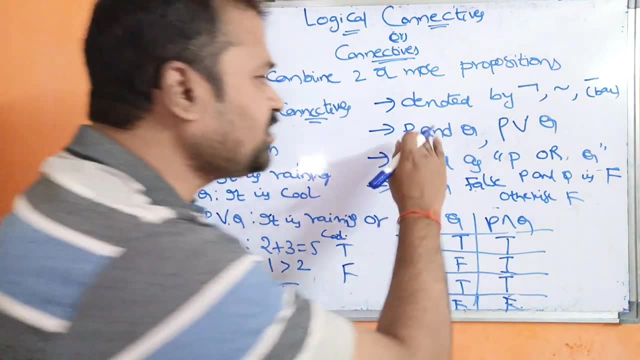 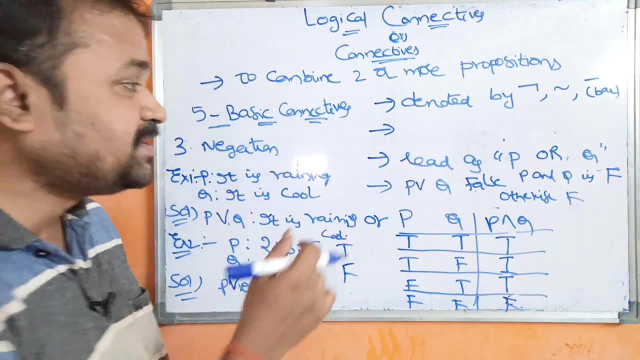 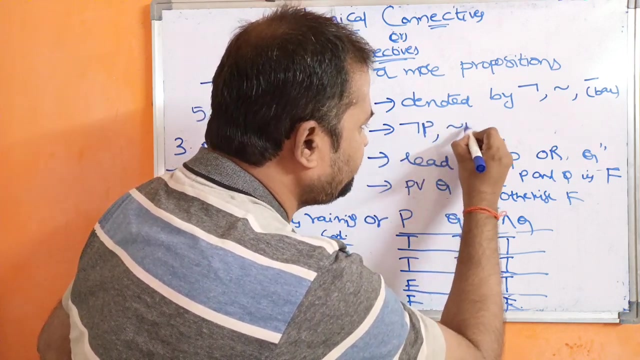 The first symbol is this one: or we can use tilde symbol, or we can use bar symbol, So this is called as bar symbol. Here only one preposition is sufficient: Here: the negation of the p, the negation of p is denoted by is denoted by negation p, negation p or tilde p or p, bar or p. 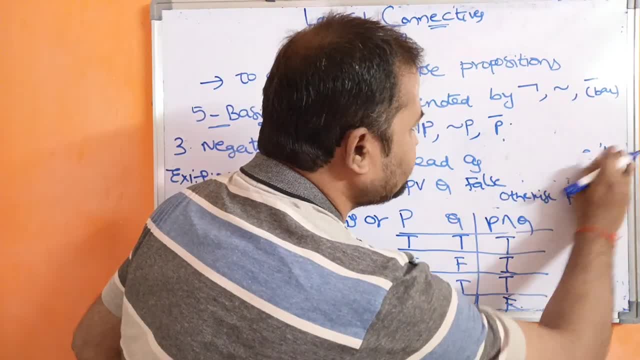 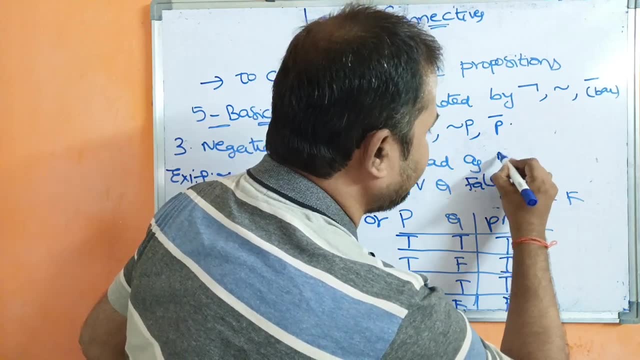 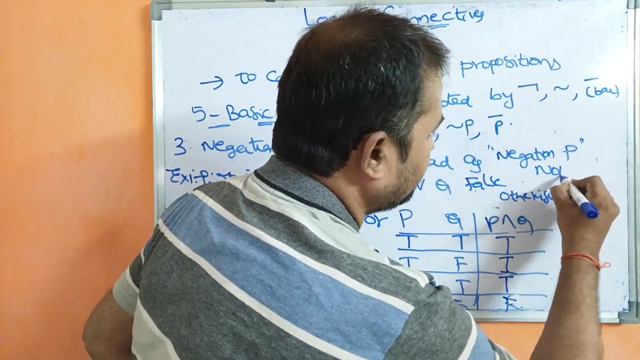 bar. So which is read as the negation of the p is read as what Which is read as p, negation of p or negation p, or we can also read it as not p, Negation p or not p which is denoted. 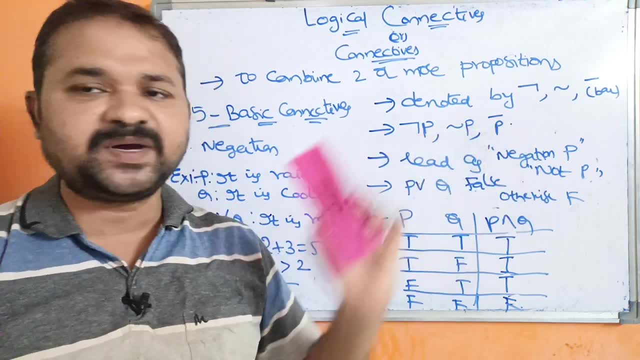 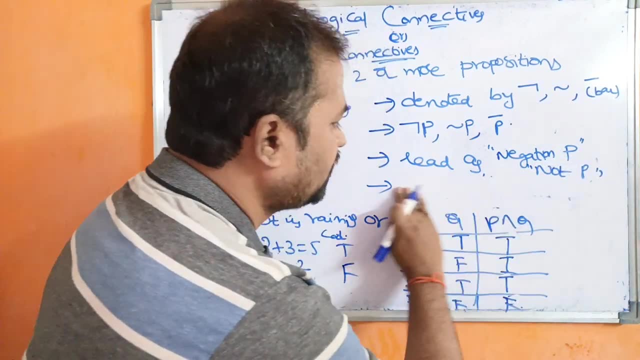 by the symbols, three symbols. We can use one of these symbol, So this can be read as negation of p or not p. Let us see what is the rule here. What is the rule here? If p is true, then negation p. 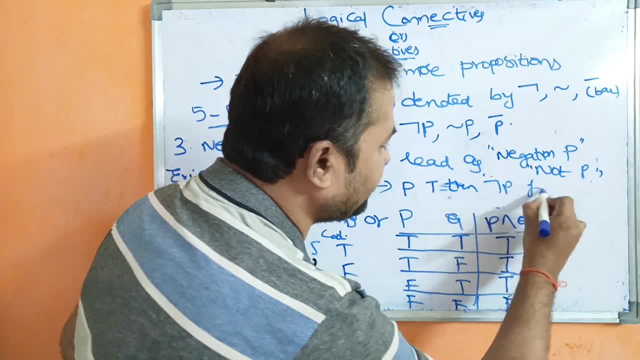 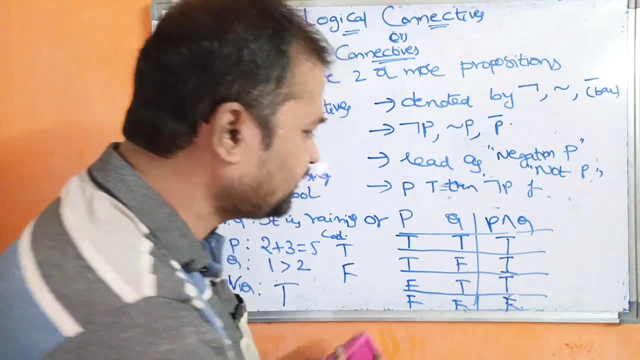 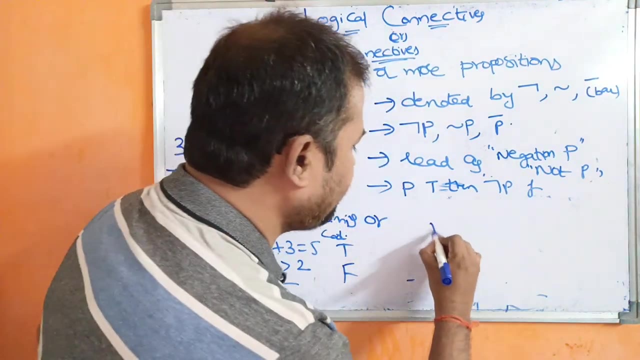 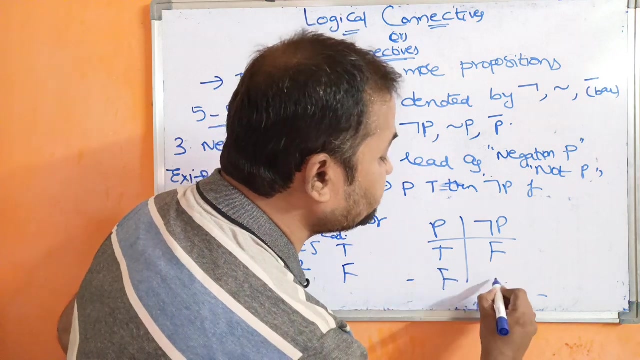 returns false value. Likewise, if p is false, then negation p returns true value. So let us see the truth table here. Let us see the truth table here. Let us see the truth table. So p, negation, p So true. If p is true, then the negation of p returns false value. If p is false, then the negation 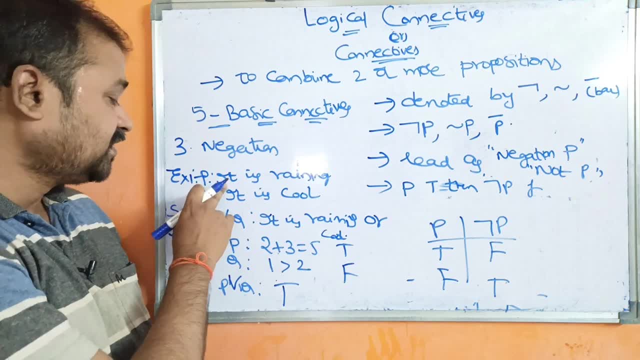 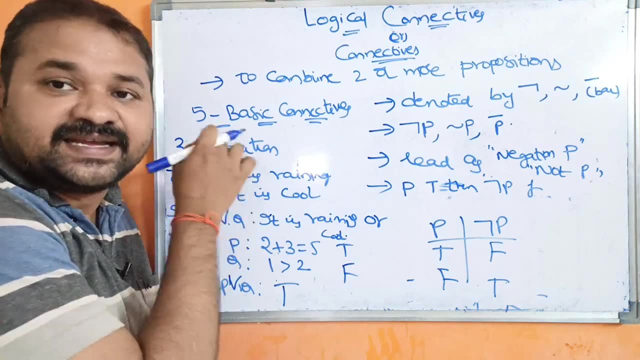 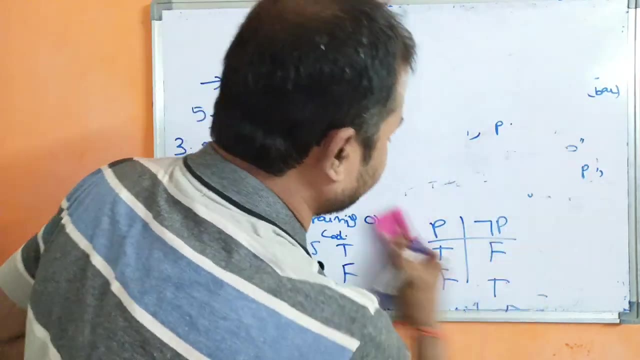 of p returns true value. Let us see an example here. Here only one preposition is sufficient. Two prepositions are not needed. Let the preposition is like this: It is raining, p, it is raining. Then negation p can be written as what It is not raining. So let us see an example for. 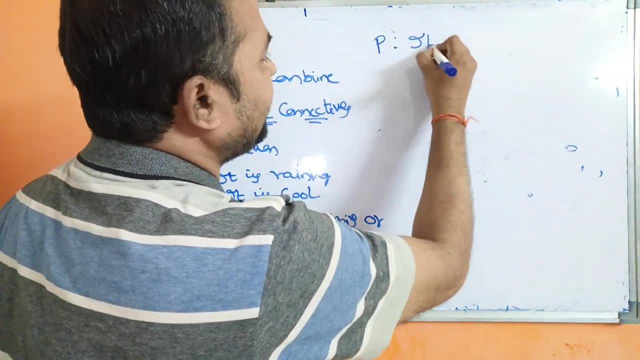 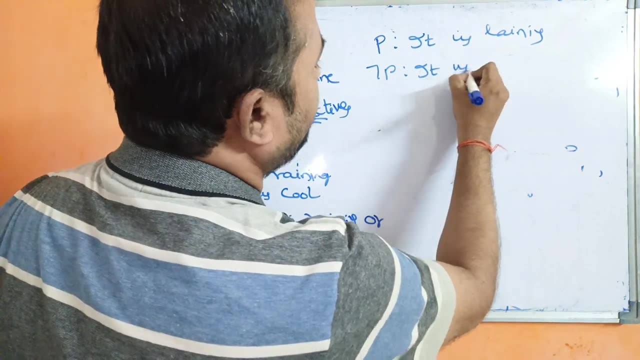 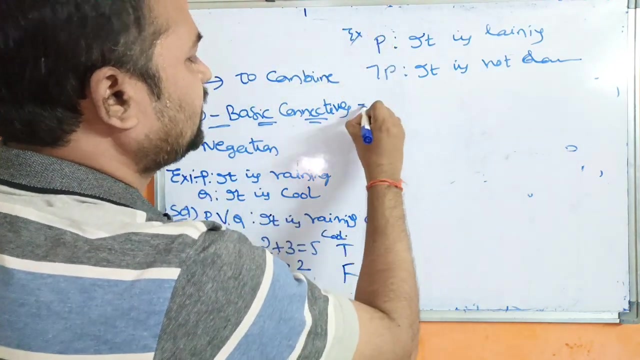 this. So p it is raining, It is raining, Then negation p is written as it is not raining. So this is nothing but negation: It is not raining. Let us see the second example. Let us see the second example. Only one preposition is sufficient. Two plus three is equal to. 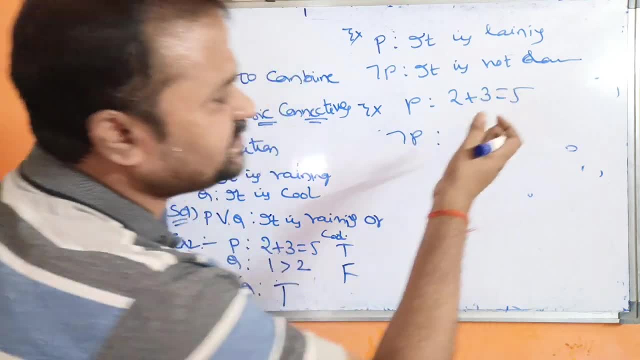 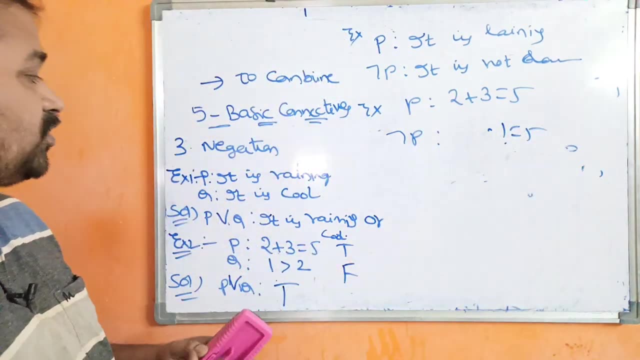 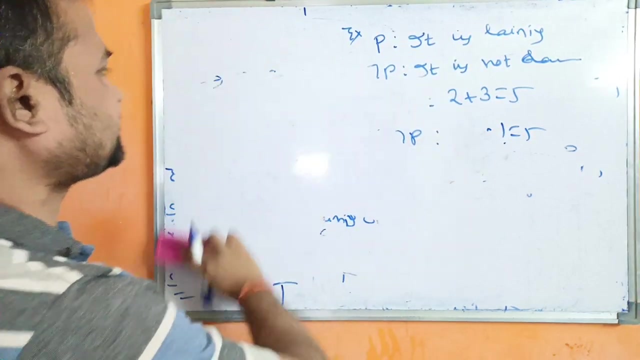 five. Then negation p means what? Two plus three is not equal to five. Two plus three is not equal to five. So this is about negation. Now let us see the remaining two prepositions. So what are the remaining two prepositions? And conditional and biconditional, So same. 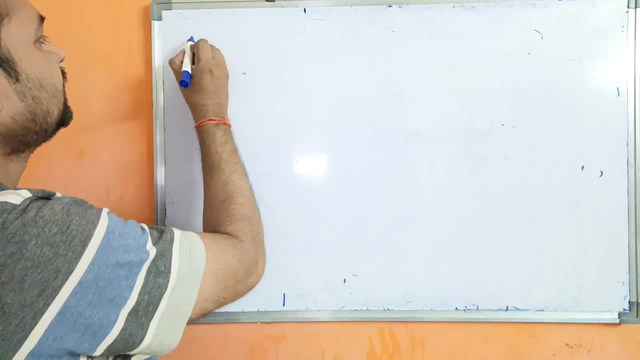 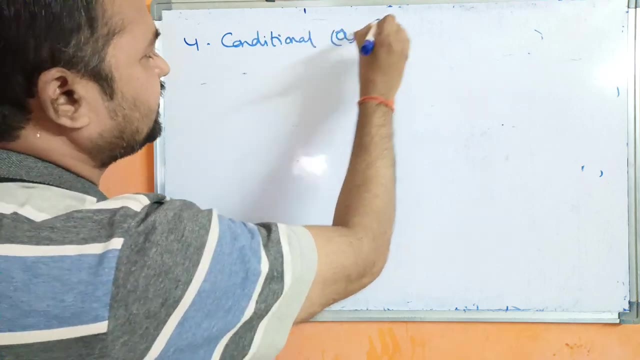 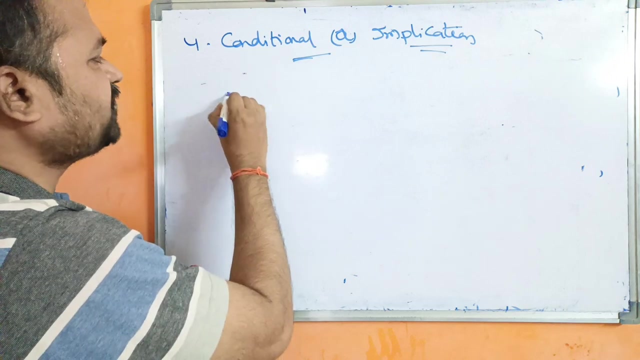 examples. So let us see the fourth one, That is, conditional. Conditional can also be called as implication. Conditional can also be called as implication. Other name for the conditional is implication. Let us see what is the symbol. The symbol for conditional is here the symbol. 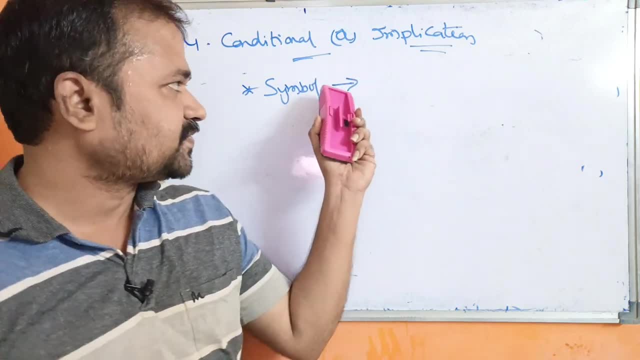 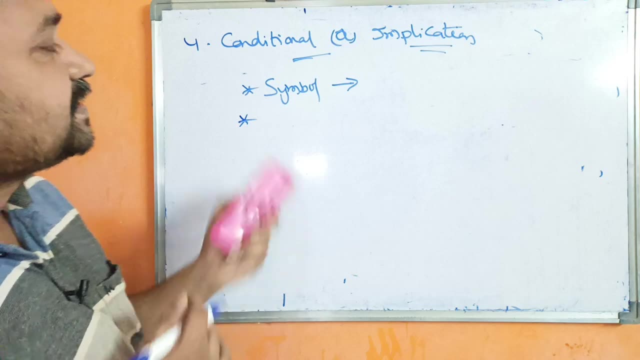 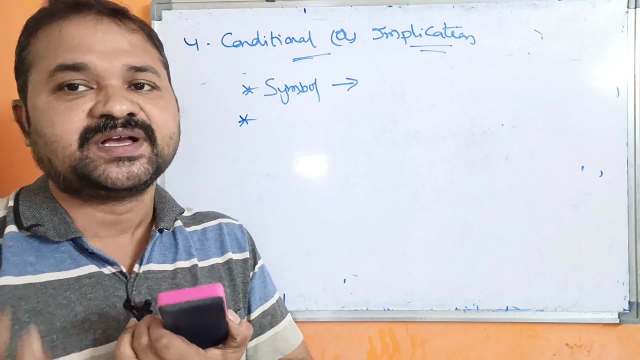 for the conditional is arrow operator, So minus greater than arrow operator. Now let us see how we can denote conditional operator Conditional. Okay, Conditional can also be called implication. The implication of two prepositions, p and q, is denoted by p? arrow. 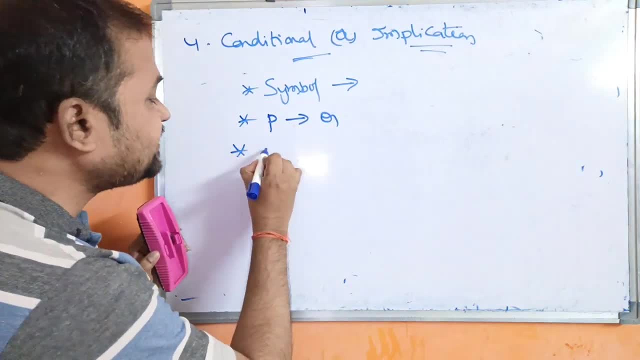 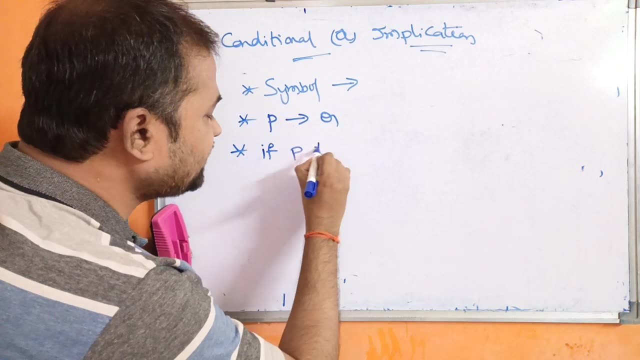 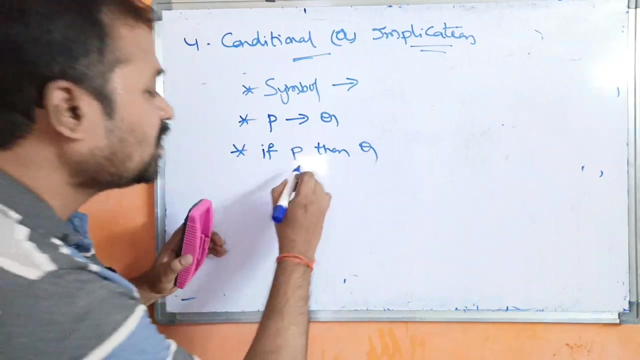 q, which is read as, which is read as: this can be written as if, if, and then if p, then q. So which is read as: p implies q, which is read as: But if p, then q, or we can write it as p arrow q. we can read it as like this: or we can read: 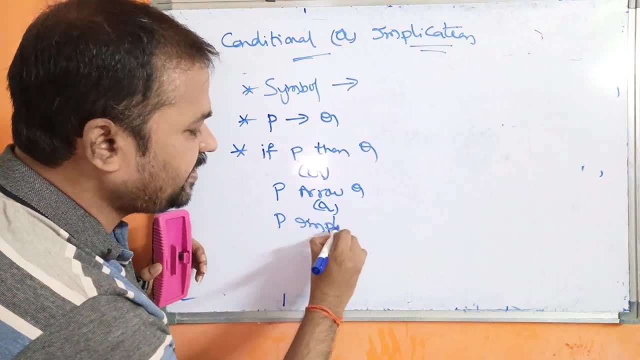 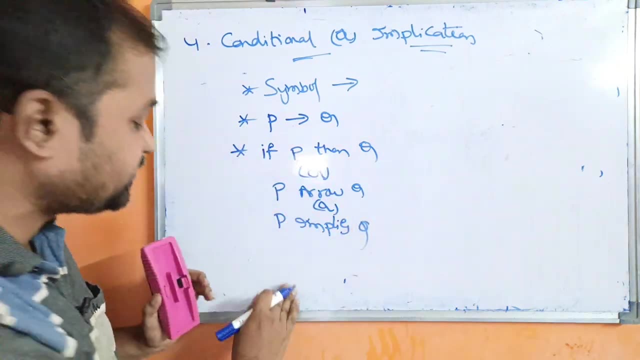 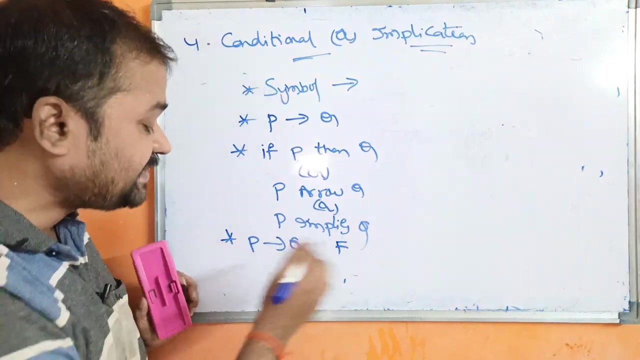 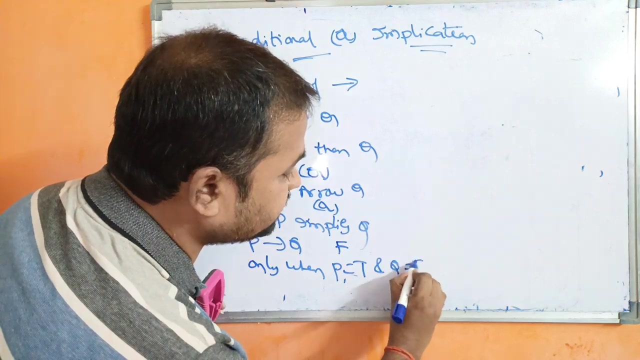 it as: p implies q, p implies q. So we can read the statement in three ways: If p, then q or p arrow. q or p implies q. Now let us see the rule here: P arrow- q returns false. It returns true and q is false. Otherwise it will returns true, only Otherwise it will returns true. 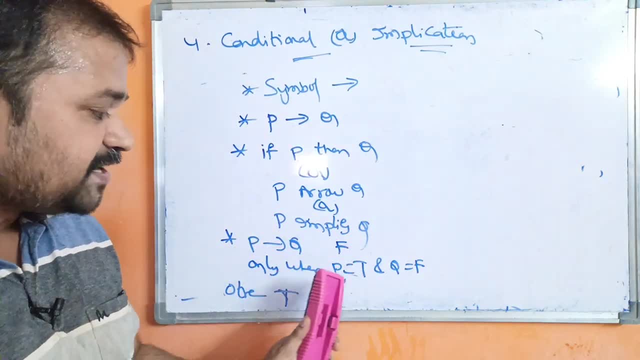 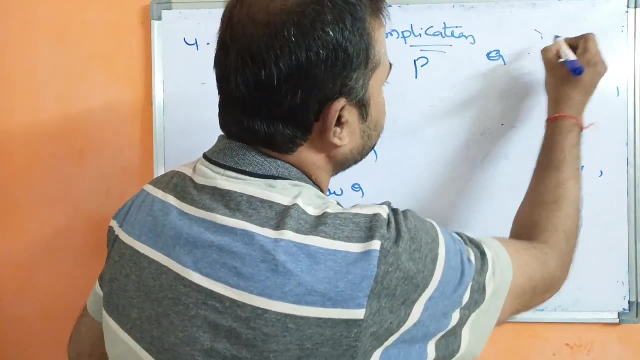 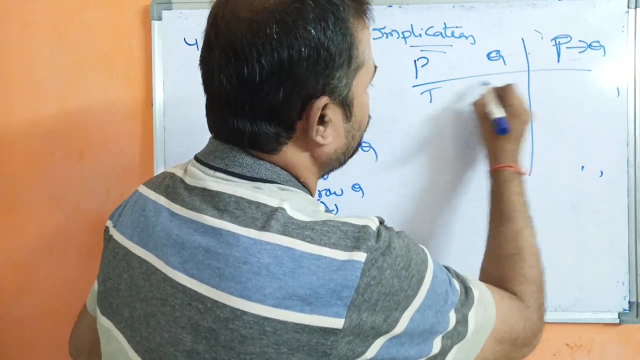 only So p and q is false only when p is true as well as q is false. Otherwise it will returns true. So let us see the truth table: So, p, q, p arrow, q, p arrow, q, So true, true, True, false. 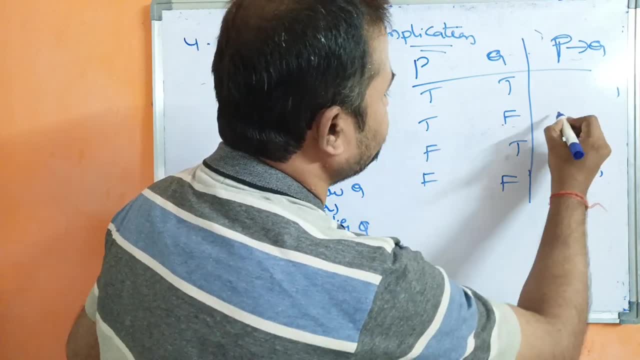 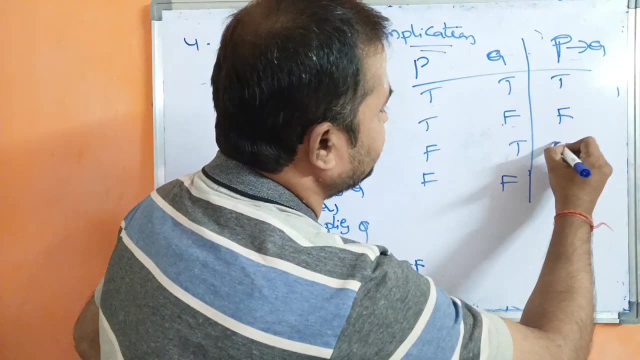 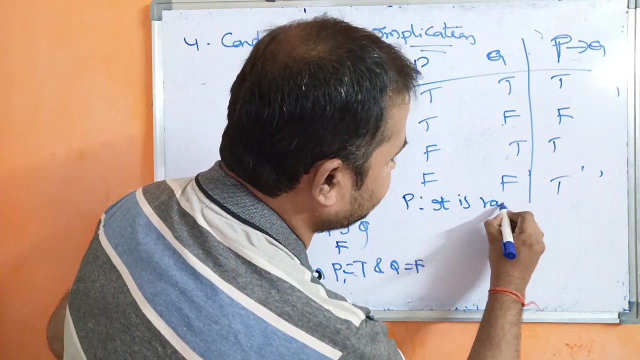 False, true, False, false. So here, true, false means false. When p is true, q is false, Then p arrow, q is false. Otherwise the result is true only Okay. Now let us see the examples. Okay, So, p same examples. It is raining, It is raining, Q, it is cool. It is cool Then. 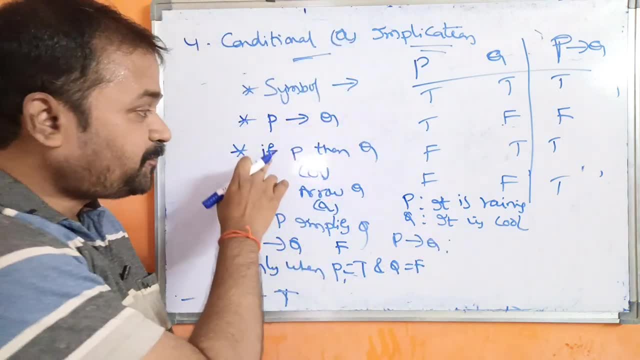 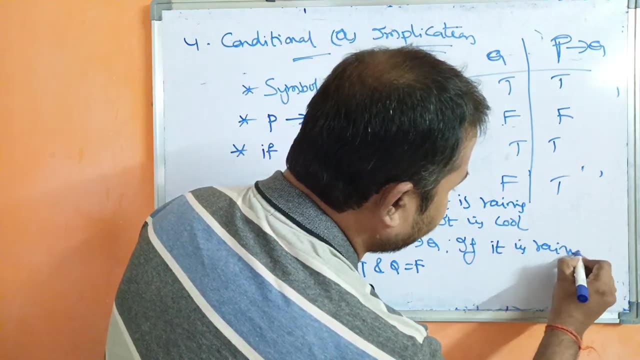 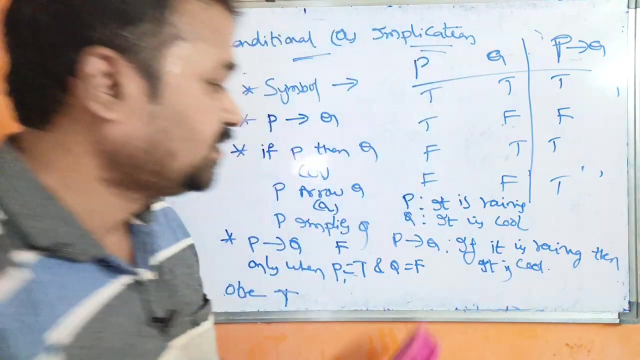 we can represent as, like this: p arrow, q. If p, then q. If what is p here? It is raining, If it is raining, If it is raining, Then it is cool, Then we can write as it also: Then it is cool, If, then? If first preposition, then second preposition, If it. 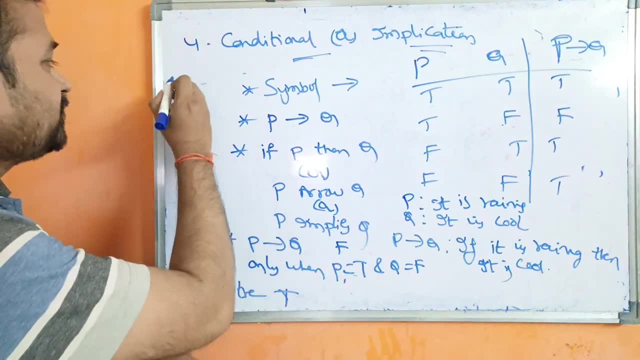 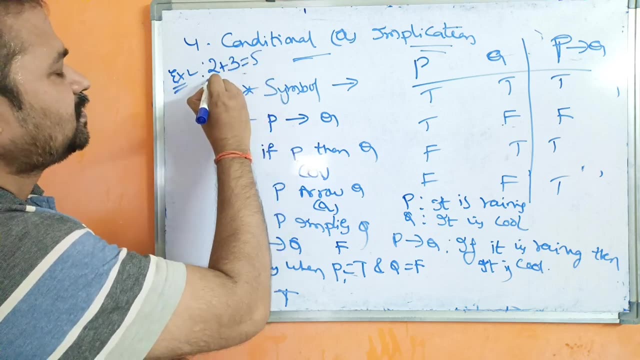 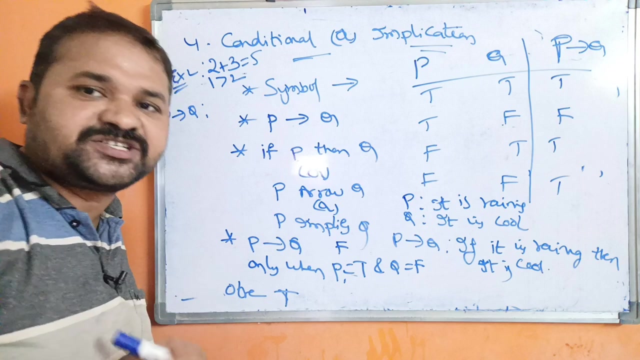 is raining, then it is cool. Let us see the second example, Example 2.. Example 2.. 2 plus 3 is equal to 5.. So 1 is greater than 2.. Then what is p arrow q? 2 plus 3 is equal to 5.. Condition is true: 5 equal to 5.. 1 greater than 2.. 1 greater. 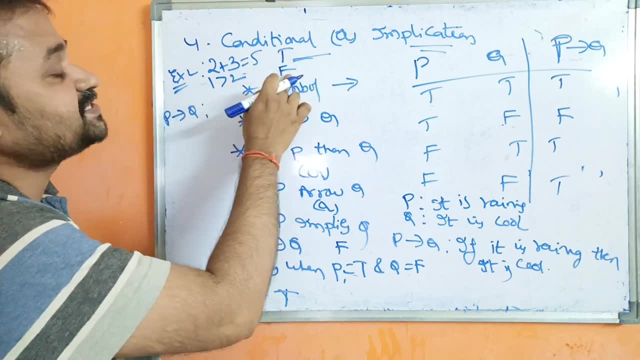 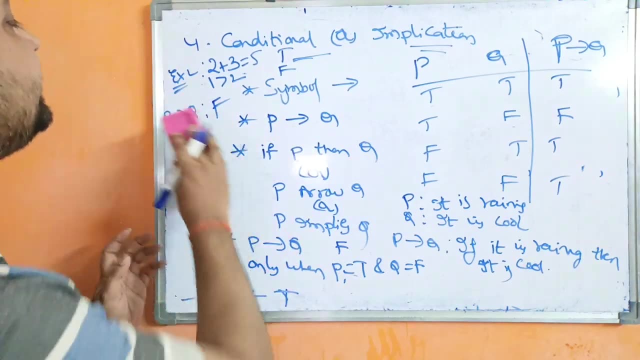 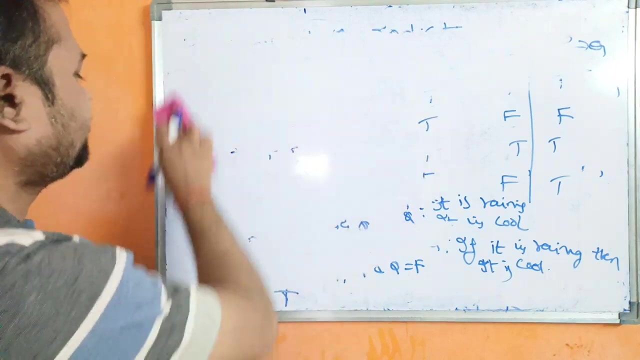 than 2.. Condition is false: 1 greater than 2.. Condition is false. True false means what False? True false means false. So this is about conditional or implication. Now let us see the last one. So what is the last one? The last one is biconditional, So the last. 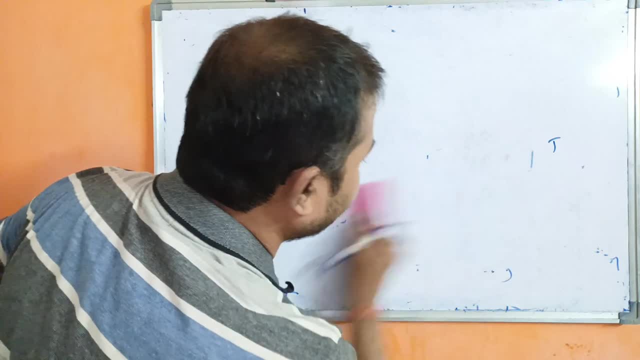 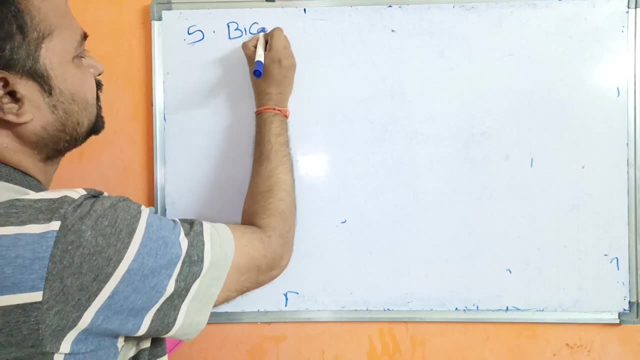 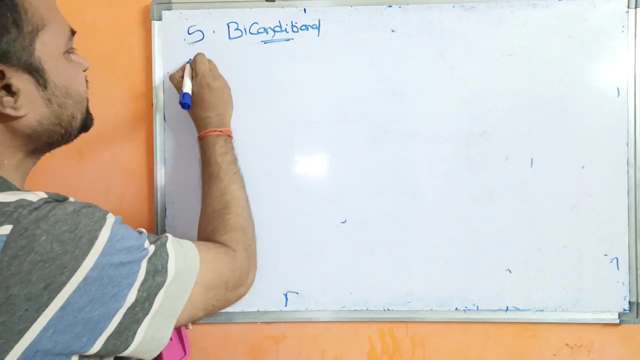 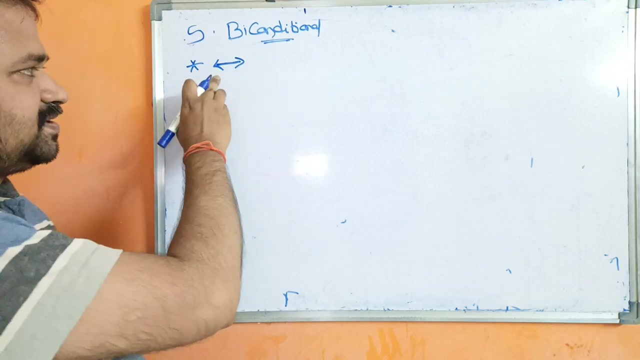 one is biconditional. So let us see about biconditional, Biconditional, Biconditional, Biconditional. Biconditional is denoted by the symbol. So, minus some horizontal line, Two arrows, we have to use Some left. 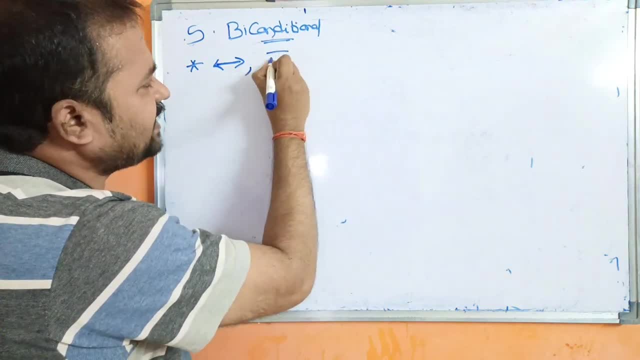 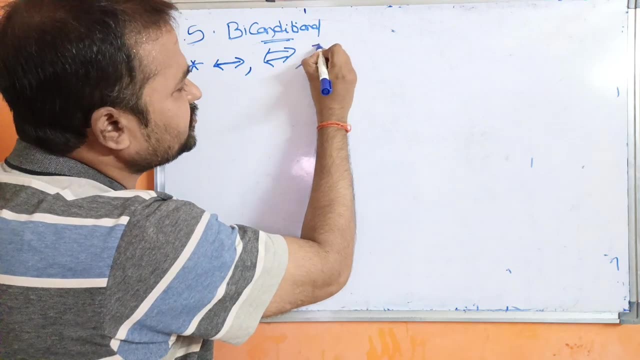 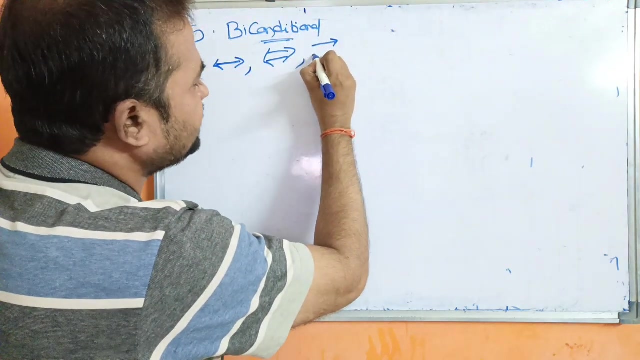 arrow as well as right arrow. Or we can use two horizontal lines. Some is equal to operator, Some left arrow As well as right arrow, Or we can use arrows like this, So some horizontal line Arrow towards the right side, Horizontal line Arrow towards the left side. Okay, So we can use. 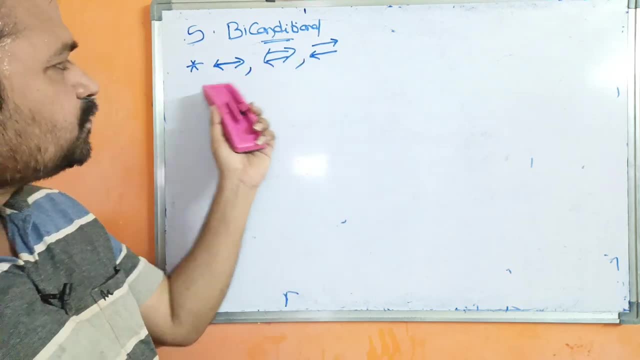 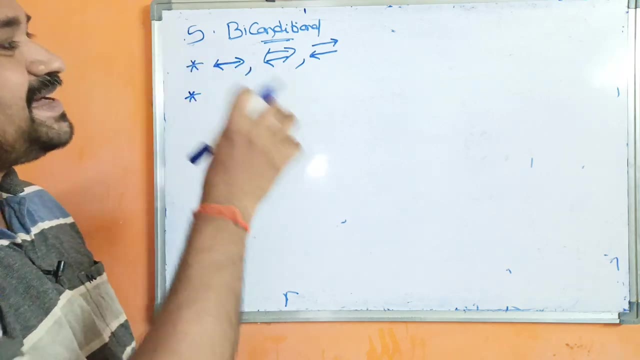 one of these symbols- Okay, Arrows should be available in both the left side and the right side. So this is about what The symbol for the biconditional operator, Now the biconditional of two propositions, p and q, is denoted by. So already we have seen. 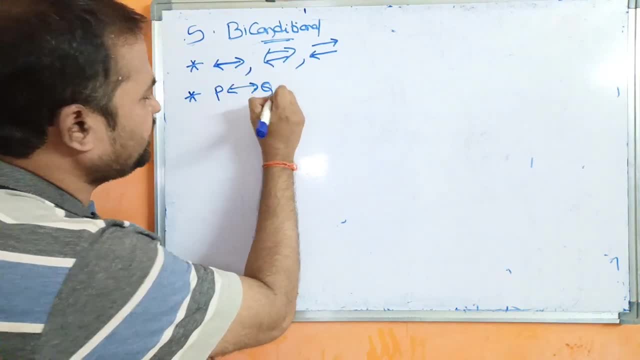 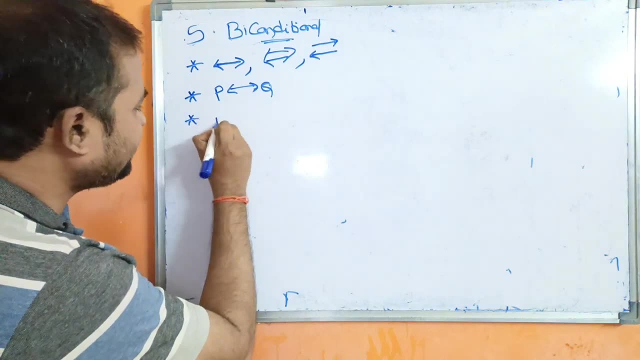 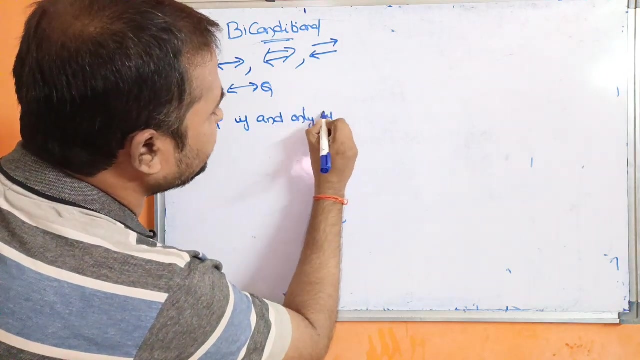 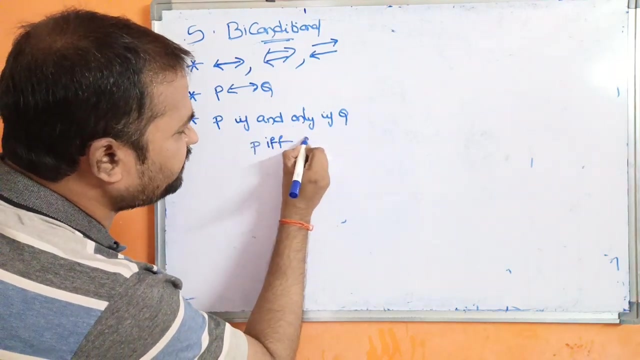 Three notations. We can use one of the notations: P, Horizontal line. Less than symbol, Greater than symbol. So this can be read as p- if and only if, q. p if and only if. q. If and only if means IFF, So which is abbreviated as p, IFF, q. So IFF stands for if and only if So. 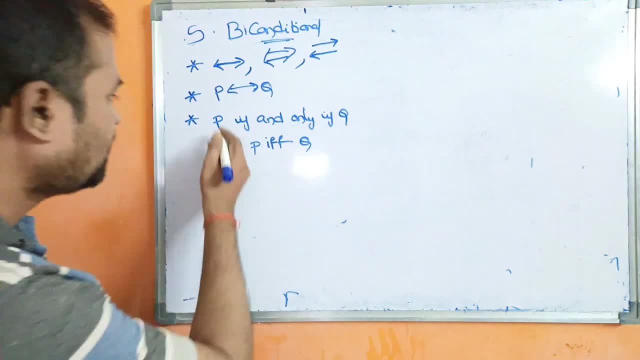 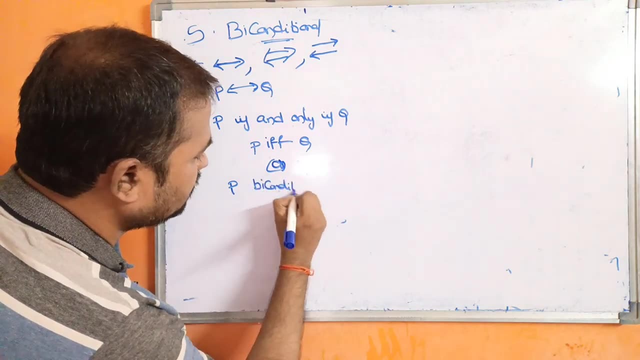 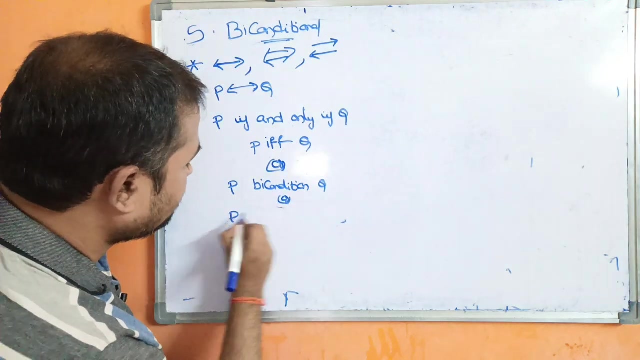 the abbreviation for if, If, and only if, is IFFF. Or we can read it as like this: Okay, P biconditional q, P biconditional q. Or we can read it as p double implies q. Why? Because we have arrows in both left side. 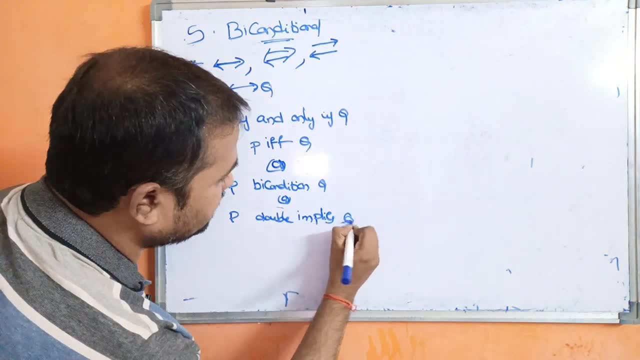 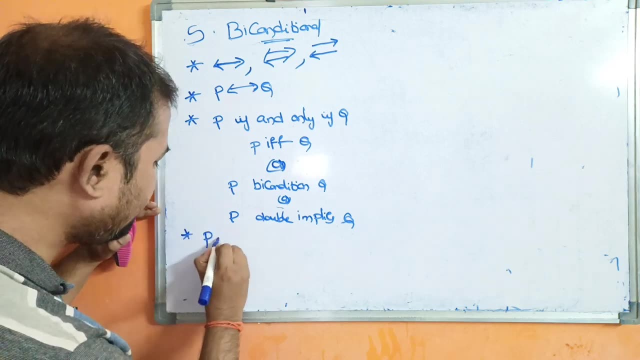 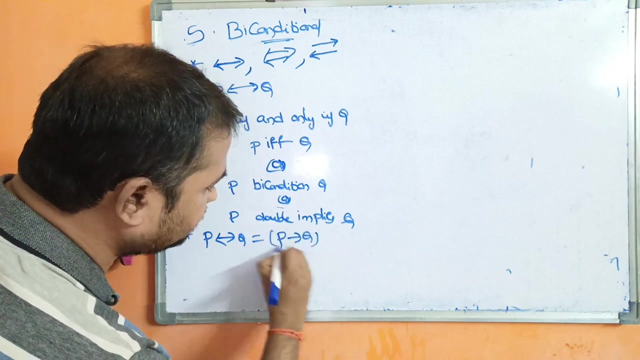 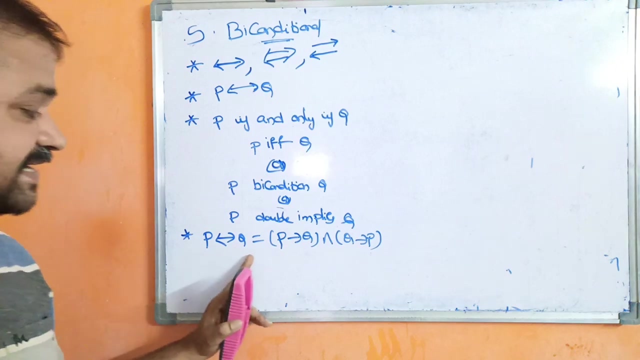 as well as right side. P double implies q, P double implies q. So in all these notations we can read this statement: P biconditional q is nothing but conjunction of P arrow, q and q arrow. p Conjunction means what And symbol. So p biconditional q is nothing but conjunction. So and So conjunction. 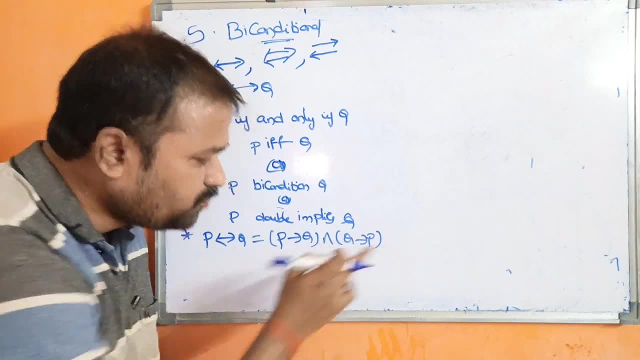 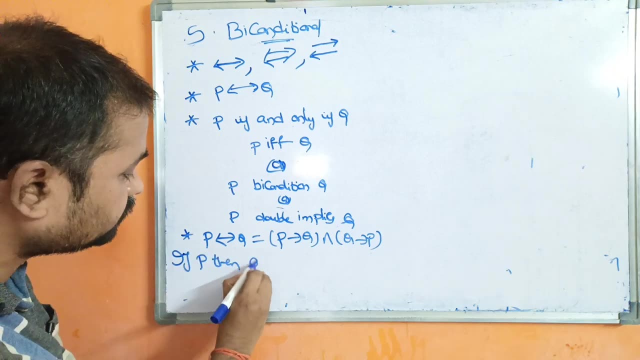 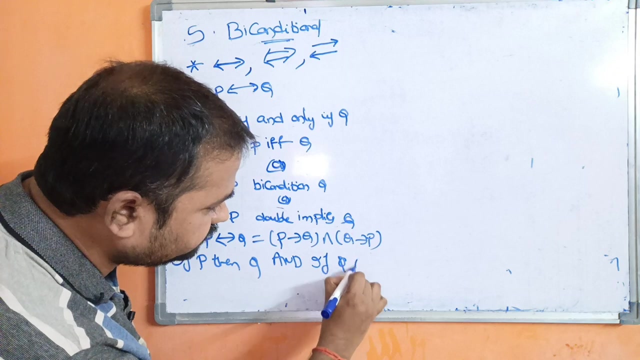 of P arrow q as well as q arrow p, So this can be read as. This can be read as: if P, then q, If P then q, And, and. so we have to use a word called and. and. if q, then p, if p then q and if q then p. now let us see. 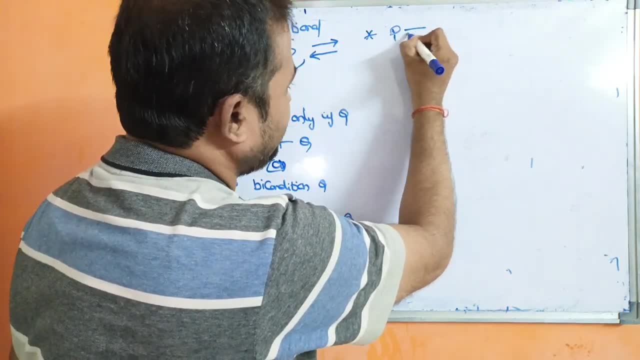 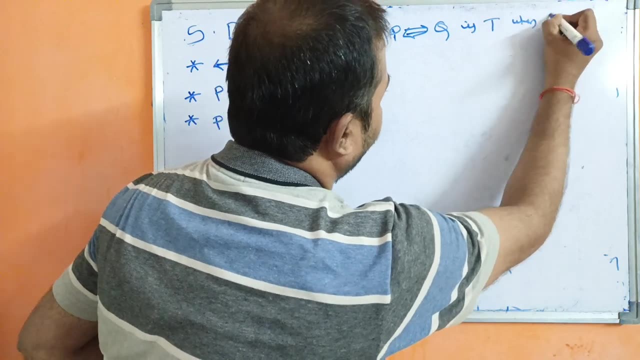 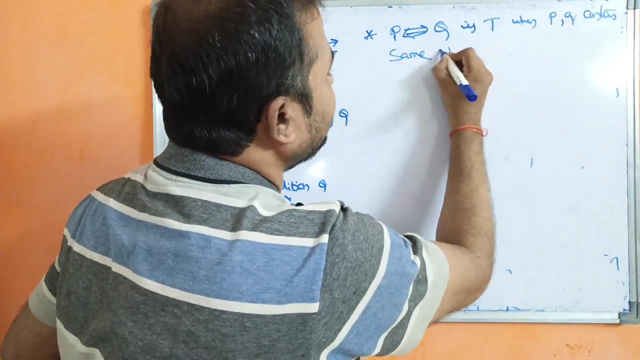 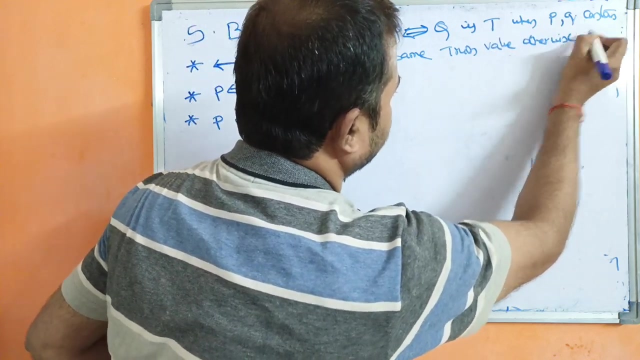 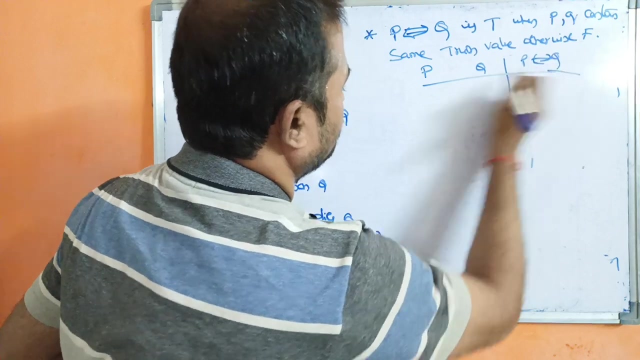 the last point, p by conditional q returns. it is true when, when p as well as q contain same truth value, contain same truth value, it may be either t true or false, otherwise it is false, otherwise false. so let us see the truth table here: p, q, p by conditional q, so true, true, true, false. 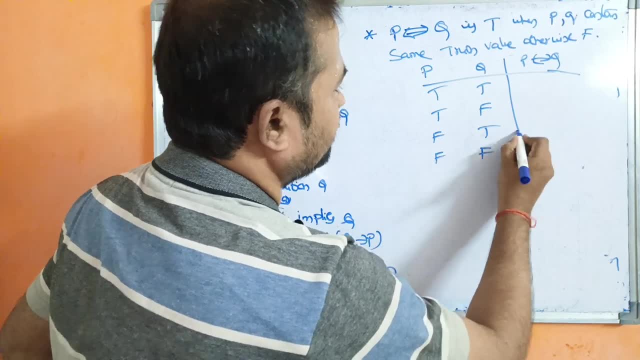 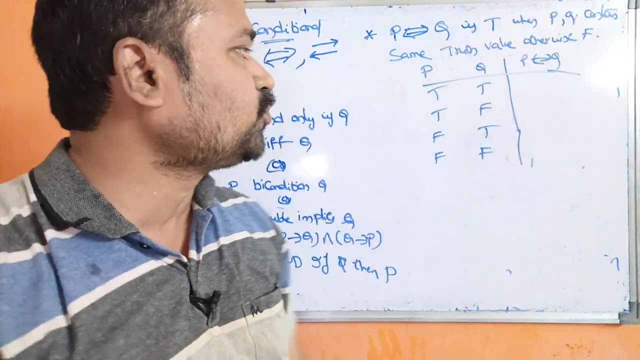 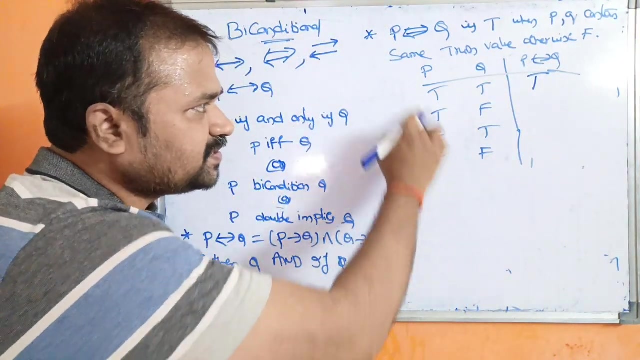 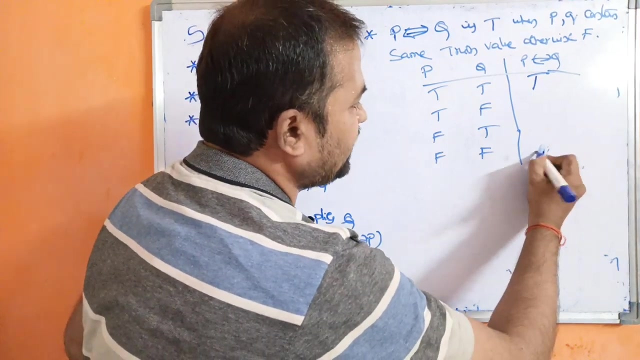 false, true, false, false. so when it will returns true, p by conditional q is true when p and q contains same truth value. here, p and q contains same truth value: t, t. so the result is true. okay, so here also, p and q contains the same truth value, that is f. so here also the result is true if p and q contain same. 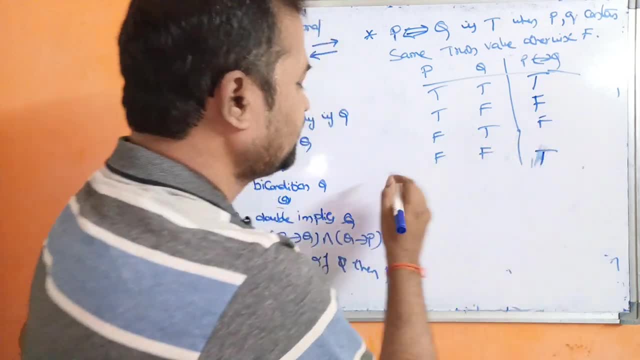 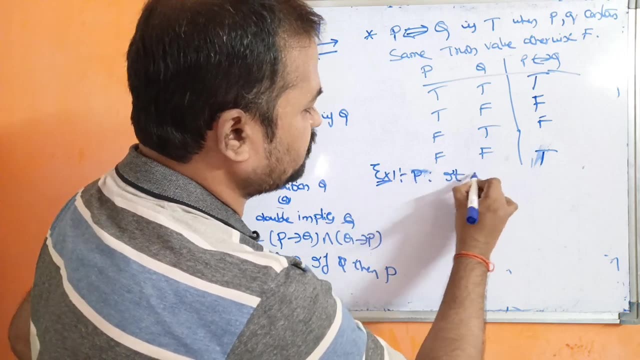 truth value, the result is true. otherwise the result is false. so let us see the example. example one: it is raining, so p. let the first preposition is p, it is raining. let the second preposition is p, it is raining. let the second preposition is p, it is raining. let the second preposition